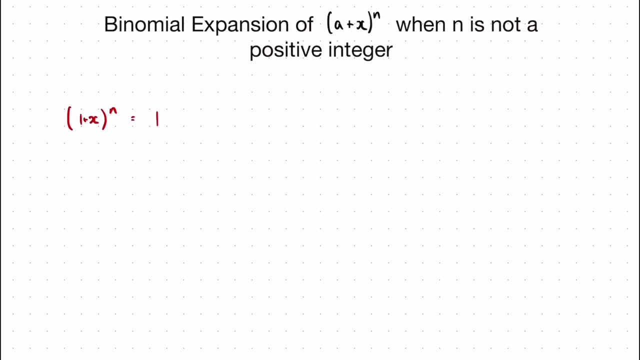 and we came up with the expansion 1 plus nx plus n, n minus 1 over 2, factorial x squared plus n n minus 1, n minus 2 over 3, factorial x cubed, so on and so forth, creating an infinite. 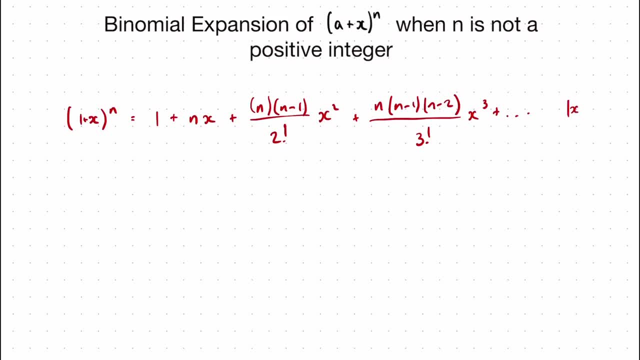 series for when Mod x was less than 1, so using this we can help ourselves generate a a plus x to the n general rule. So the first thing to consider is that a plus x to the n can be rewritten as in its factorised. 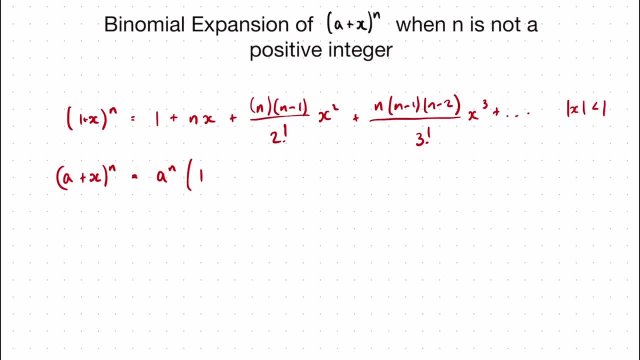 form of a, n, 1 plus x over a to the power n. So all we've done is factorise a out of the bracket, and when you factorise a out of your bracket, like so with power n, then you can expand this other bracket to get to this generalised. 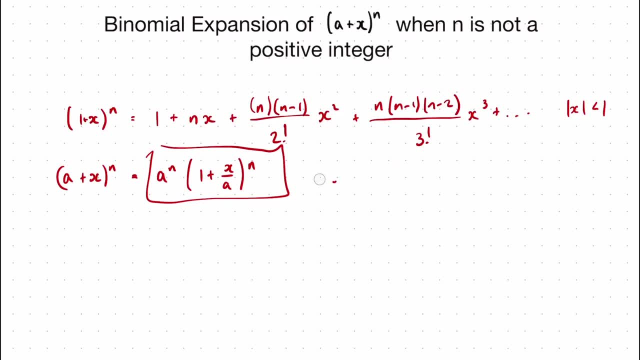 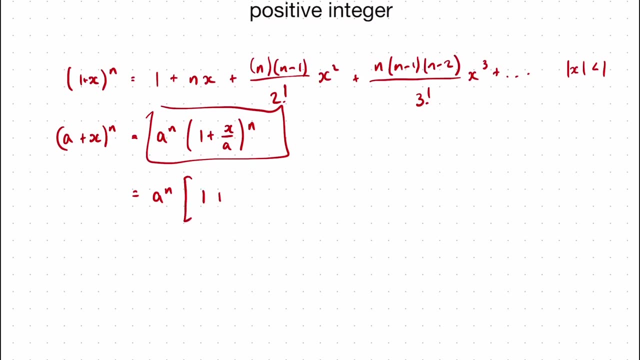 writing. So using that we can expand similarly to the 1 plus x to the n, n minus 1 over 2. factorial is e to the n Sheed to the play after Now we've also added an expansion to the original, so this time we are going to try. 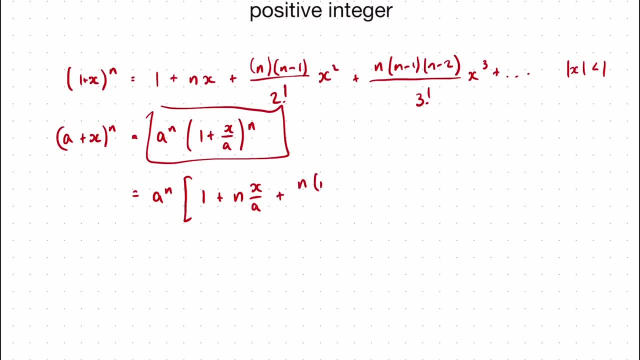 and see what this actually means If you come to the herAcademycom website with some солн". If this is your example and you day go forward and you still don't like it, then I suggest that you try this. If you briefly. 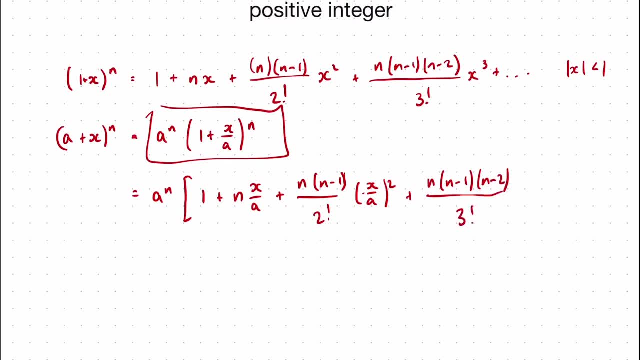 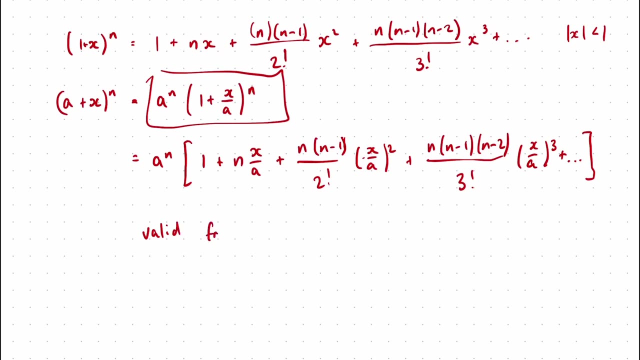 Maybe 2 over 3, factorial x over a cubed, and again so and so forth, infinite series. but this time this is only valid for when x over a is less than 1.. So, similarly with the previous lesson, when the x became a 2x squared, it became mod 2x. 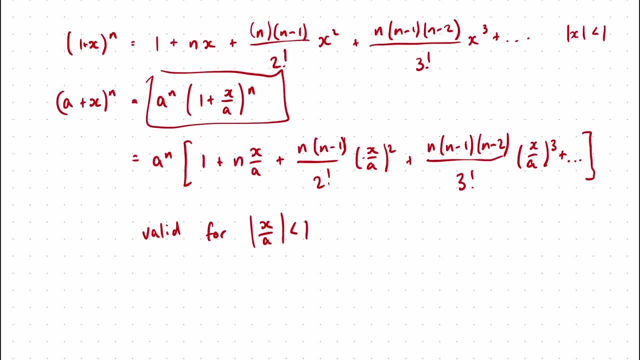 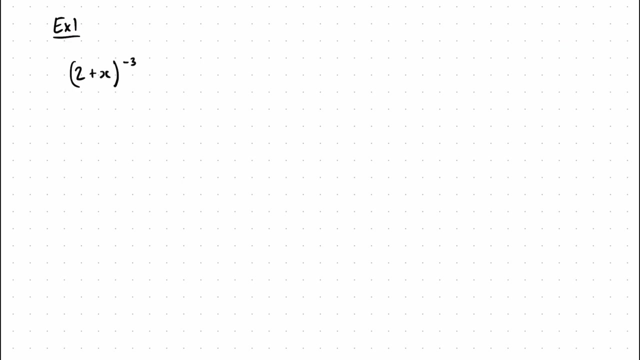 squared is less than 1, because our x is now x over a, it's now mod x over a is less than 1.. So using this, like we did with the 1 plus x to the n, we can solve questions. well, solve questions like this one here, which is expand 2 plus x to the minus 3 in ascending powers. 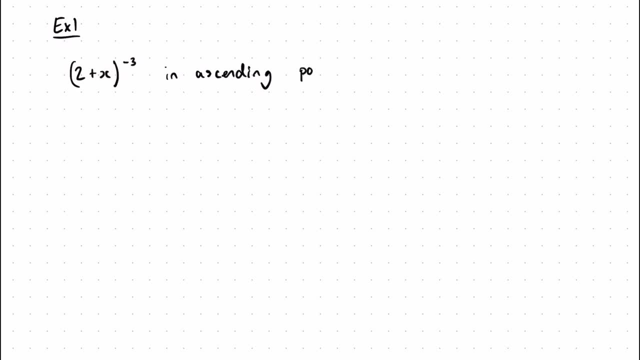 okay, Up to and including x cubed and state the range of values of x for which it is valid. okay, so, range of values of x for which the expansion is valid, for which it is valid. Okay, so, let's have a go at that now. so 2 plus x to the minus 3 can be rewritten as: 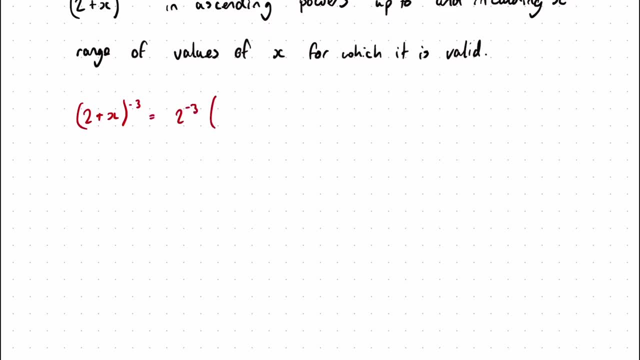 2 to the minus 3, 1 plus x over 2 to the minus 3. and then we will expand this 1 plus x over 2 to the minus 3 into its infinite series, and say 2 to the minus 3 times 1 plus n, which. 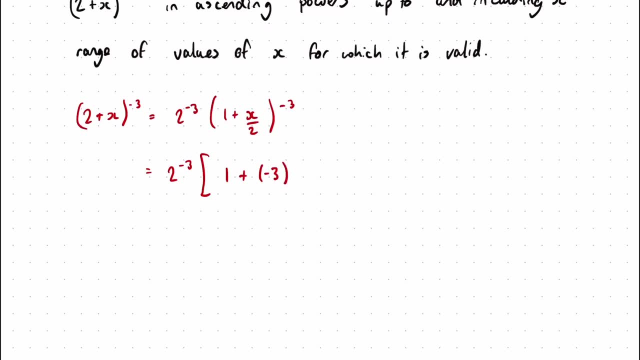 is minus 3. x is now x over 2 plus n, n minus 1, so minus 3 minus 3 minus 1 over 2 factorial times. x over 2 squared plus n, which is minus 3, n minus 1, n minus 2 over 3 factorial times. 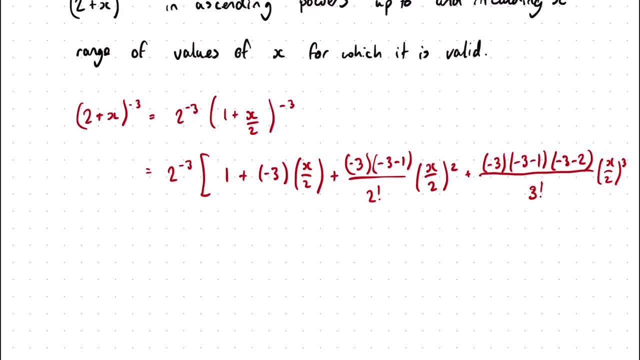 x over 2 cubed, and this would carry on again infinitely, but it we only want to go up to the powers, including x cubed, which we will have got here with that x over 2 squared. Okay, Okay, Okay, Okay Okay. 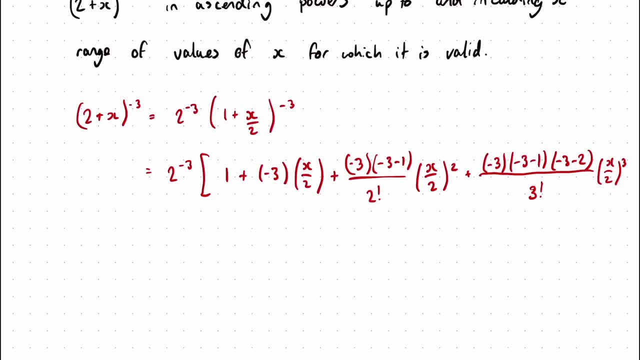 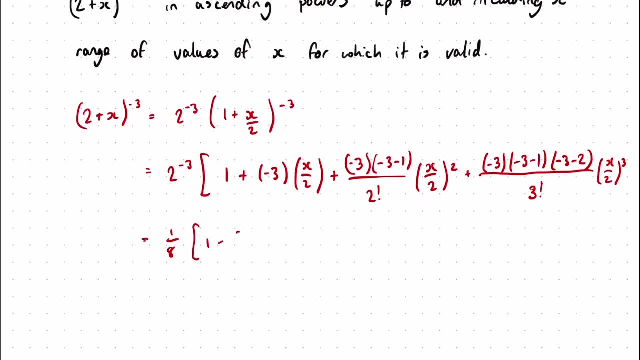 going to give us, in our bracket, 1 minus 3 over 2 x plus 3 over 2 x squared, minus 5 over 4 x cubed. Okay, so on and so forth, which, when expanded again with our 1 eighth, is going to give us 1 eighth minus. 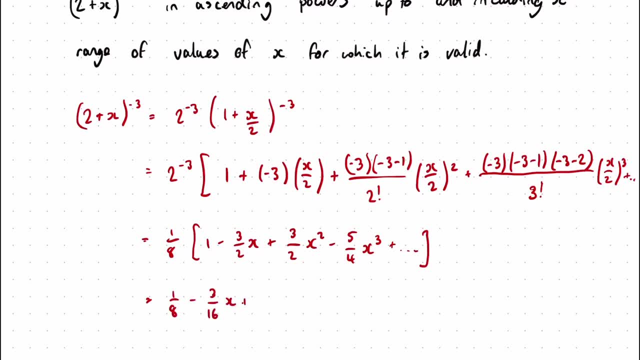 3 over 16 x, plus 3 over 16 x squared, minus 5 over 32 x cubed, so on and so forth. so that's our full expansion. lastly, we want the range of values of x for which it is valid. so that is when we take our x divided by our a. 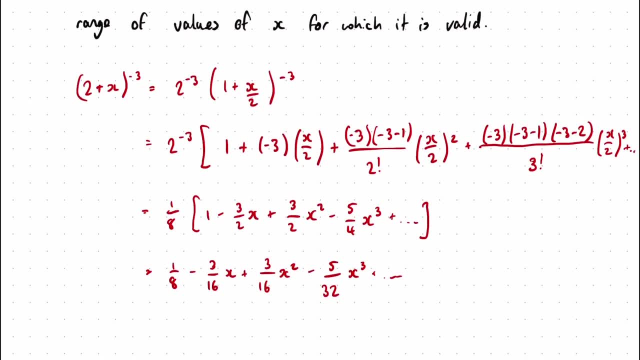 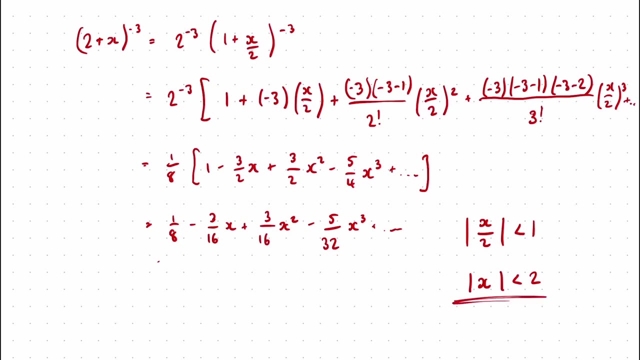 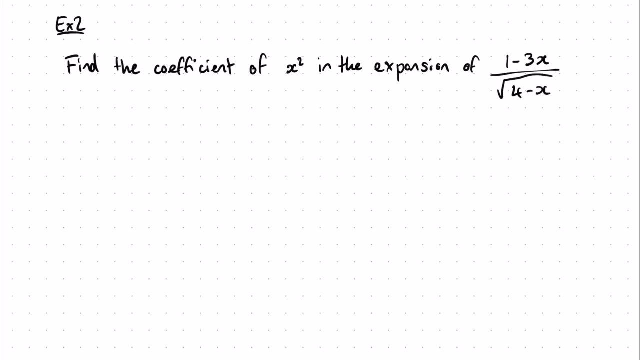 and say is less than 1. so that is for when mod x over 2 is less than 1, which is when mod x is less than 2. so these are our answers valid. let's have a look at another question. so example 2 is: find the coefficient of x squared. 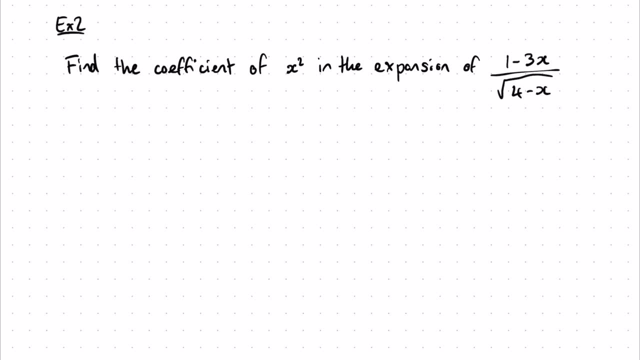 in the expansion of 1 minus 3 x over root 4 minus x. to do this, you're first going to have to get rid of the fraction and the root sign and change them to powers so we can rewrite 1 minus 3 x over root 4 minus x. 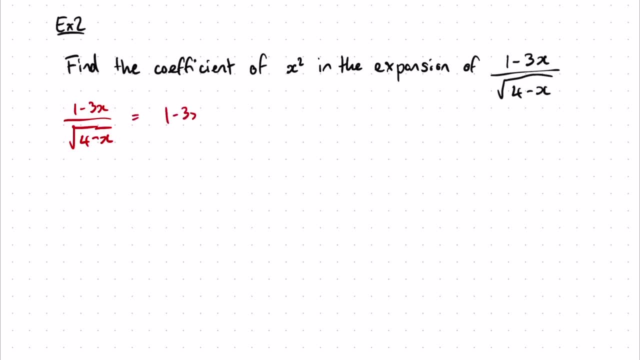 as 1 minus 3 x multiplied by 4 minus x, to power minus half. ok, so get rid of a fraction by negative power, get rid of the root sign by putting it to power half. Okay, now we need to consider our expansion. what this will become as 1 minus 3x multiplied by factorizing. far out of this. 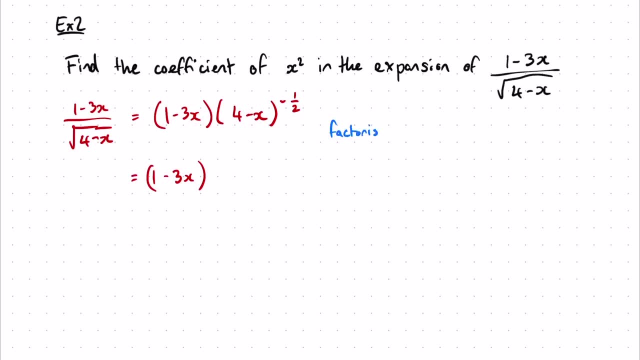 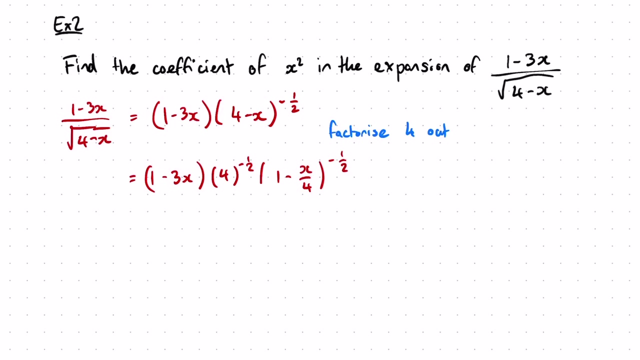 So we're going to factorize far out, which will give us 4 to the negative half, multiplied by 1 minus x over 4 to the minus half. Okay, so then we can expand 1 minus x over 4 to the negative half into its infinite series. 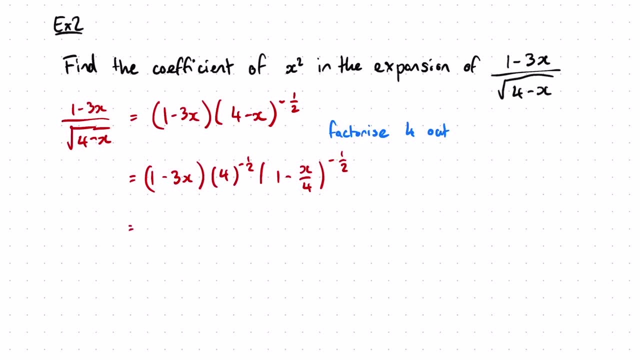 And write this all as one thing. So 4 to the minus half can be rewritten as a half. That's going to multiply by 1 minus 3x times the infinite series of 1 minus n, which is minus a half times our x, which is minus x over 4.. 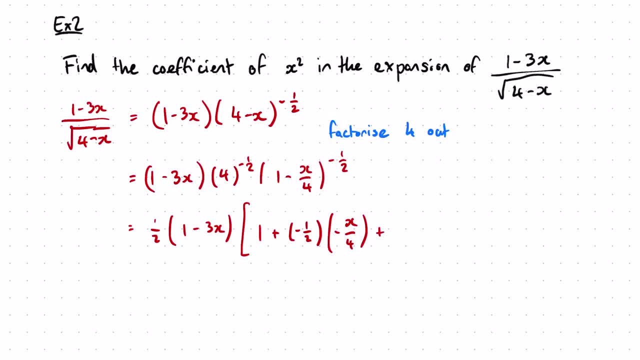 Plus, sorry again, that should be plus n, n minus 1.. So that's minus a half, minus a half, minus 1 over 2 factorial times, minus x over 4 squared. And I don't need to carry this on anymore because I'm only trying to find the coefficient of x squared. 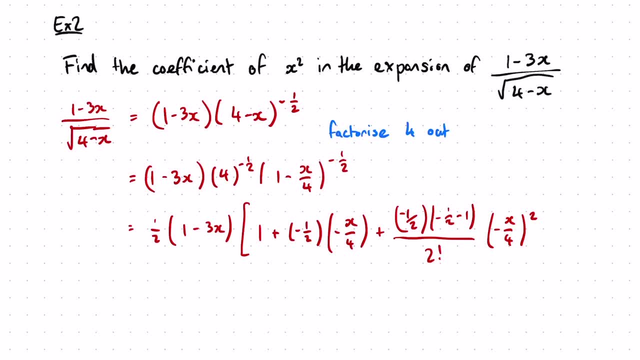 And the coefficients of x squared are going to be generated when I multiply this infinite series By the bracket, which will give me the two multiplications that I need to consider, which is the 1 times the x squared term and the x times the x term, because that will also give me an x squared term. 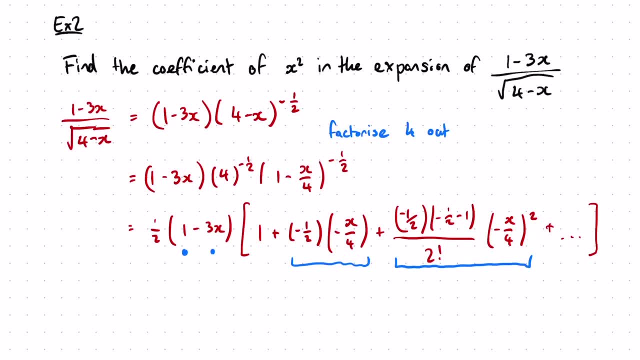 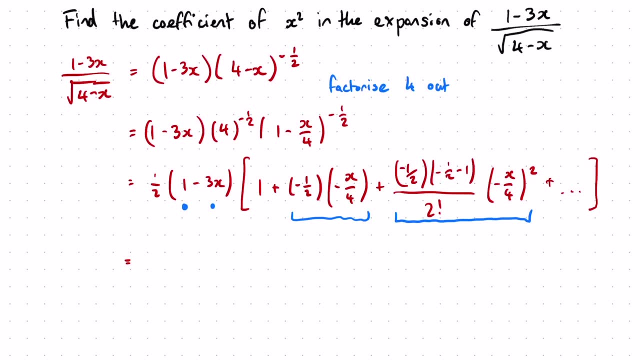 So one of the ways to do this would be to first consider half 1 minus 3x as a single bracket, So I can rewrite this as: So I can rewrite this as A half minus 3 over 2x, And then also simplify down these terms to begin with, which will give me 1 plus 1. eighth x plus 3 over 128 x squared plus so and so forth.